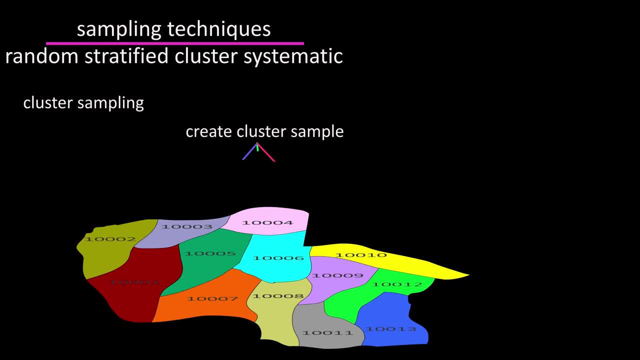 So you could create a cluster sample using zip codes and maybe survey two or three of the 13 different possible zip codes. Cluster samples can be efficient and cost-effective. However, there are times when the cluster does not represent the population. A little note the main difference. 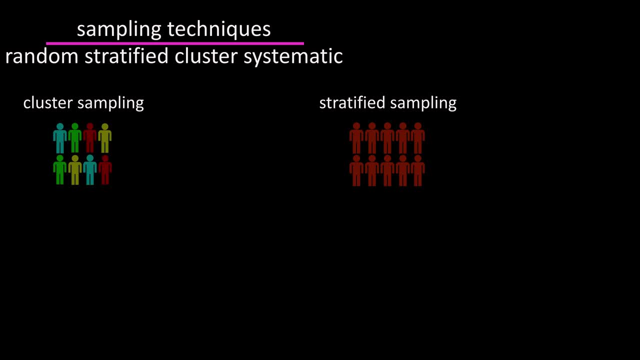 between cluster samples and cluster samples is that the cluster does not represent the population. The reason for the difference between cluster samples and cluster samples is that the cluster samples are identified by the individual and the individual in the cluster. The difference is that subgroups in the stratified sample have similar characteristics and the subgroups or clusters in 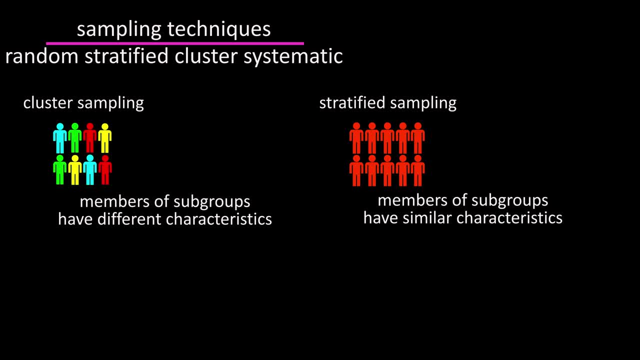 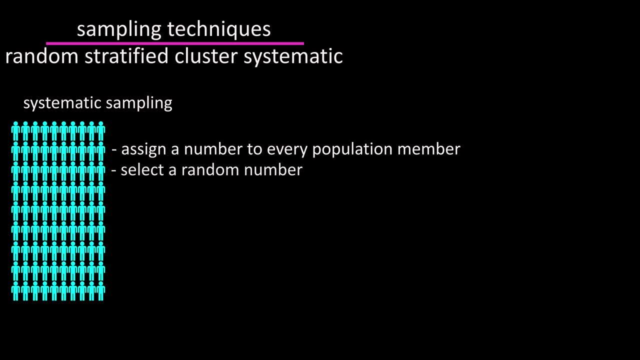 the cluster sample are intended to vary in characteristics. A systematic sample is where a researcher will assign a counting number to every member of the population, then select a random number, then select members for the sample at regular intervals from the starting random number that was selected. For example, let's say you wanted to know how much time people living in 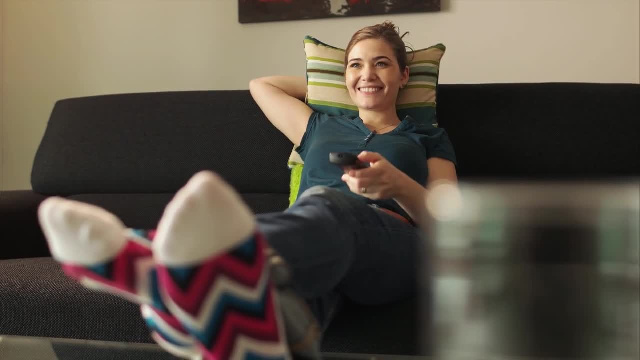 a singles-only apartment complex would take to count. If you had a number, that would be the number that you would select, then you would want to know the number- that would be the number, that would be complex- spent watching Netflix on a weekly basis. You would want to get, say, a sample of 50 members. 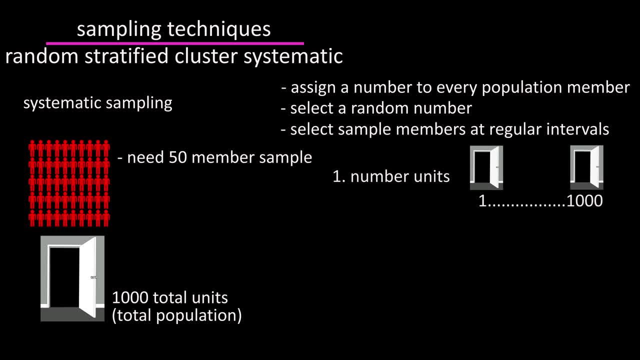 If there were a thousand units in the complex, you could number the units one to a thousand and generate a random starting number, say 234.. Since you want a sample of 50,, you could divide 1,000, the number of the population by 50 to get 20, which would be your interval number, So 234. 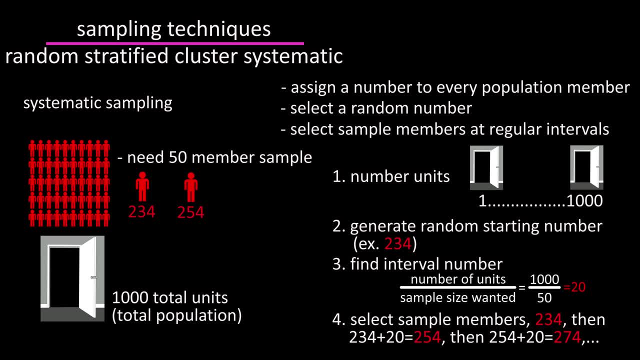 would be selected for the sample, then 254,, which is 234 plus 20,, then 274,, which is 254 plus 20, and so on until you had your 50 members selected for your sample. This sampling method is easy to. 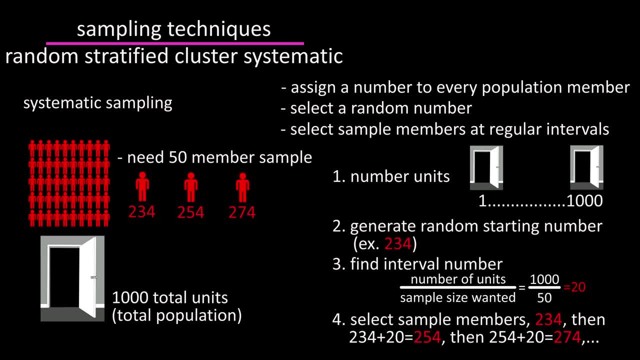 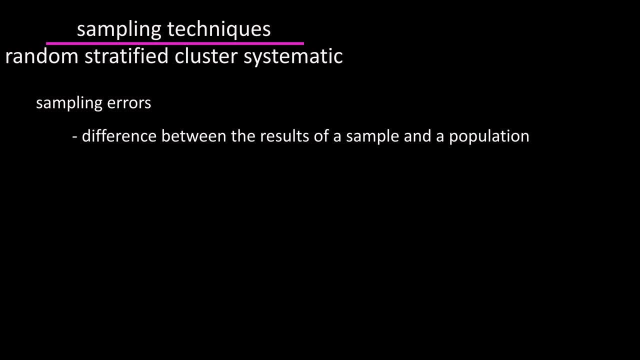 use if the population can be easily numbered. Another note: even when using the best sampling methods, a sampling error, which is the difference between the results of a sample and a population, can occur. And there is one other sampling method, called a convenience sample, where a researcher 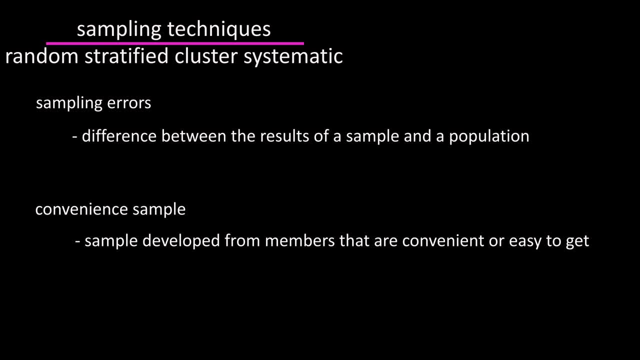 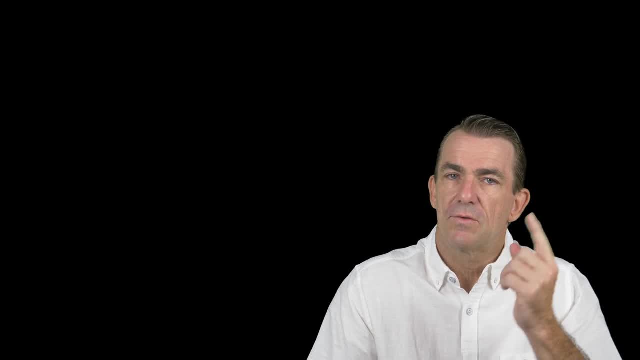 developed a sample of a population and then used it to calculate the number of members. A sample develops a sample from members of the population that are easy to get or convenient. Many times, these samples lead to biased results. All right, my friends, I have more videos, right? 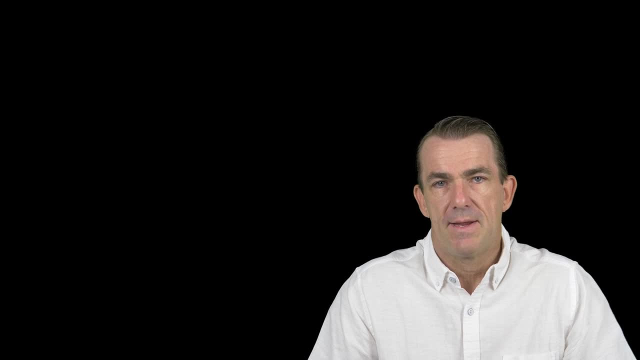 there for you Till next time I am out of here.